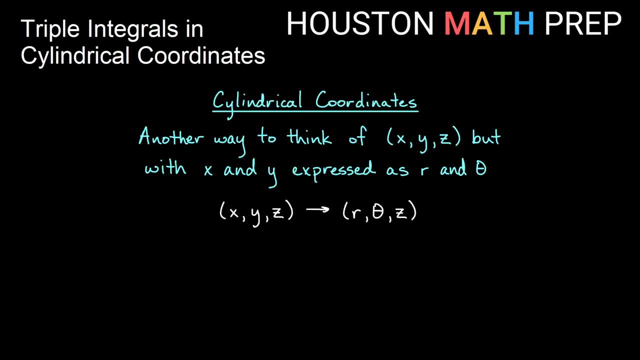 thought of as r and theta instead. So we're not going to change z. Z still is going to be this vertical component that we think of in three-dimensional space, but when we have some sort of a round type of solid or region, we want to think in terms of polar. perhaps Might be a. 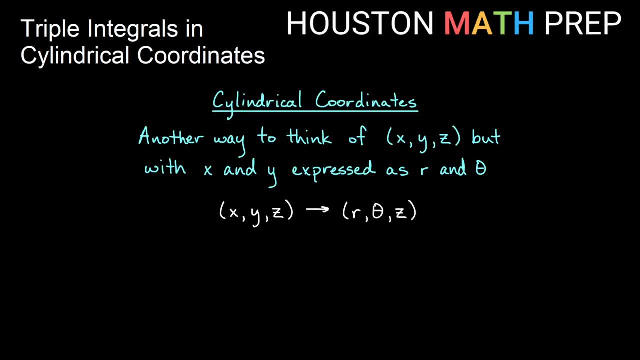 little easier to deal with formulas than in terms of x and y and z. So our coordinate system will be based on r and theta and z. So if we have some point in 3d space, remember that r is just going to be the distance out in the plane from our origin or from our pole. when we think of the plane. 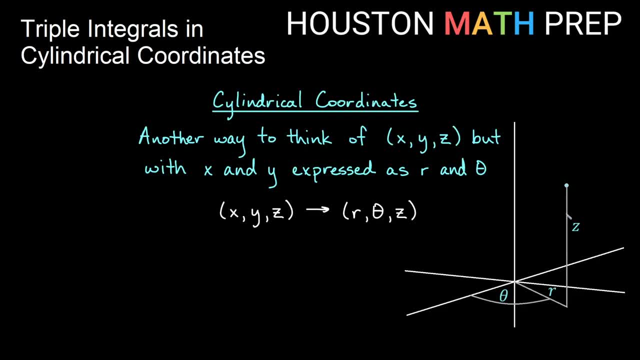 So the idea here is: we may have some height now z in the plane. We may have some height now z in the plane. We may have some height now z in the plane, three-dimensional space, where in polar we were just in the plane. So really r you can think of. 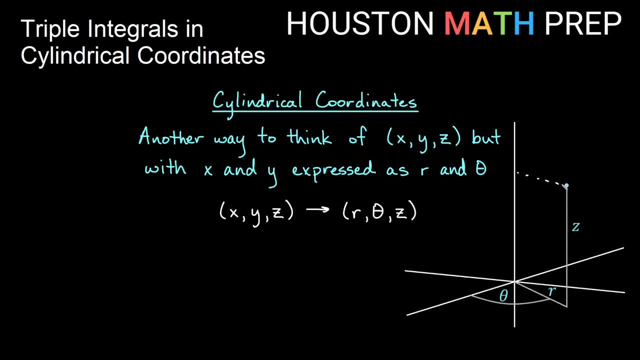 as the distance out from the z-axis to the point- Whether you're thinking underneath the point in the plane or you're actually thinking straight up from the axis. r is going to be that distance out from the z-axis- Our theta is thought of in the typical xy plane, measured counterclockwise from. 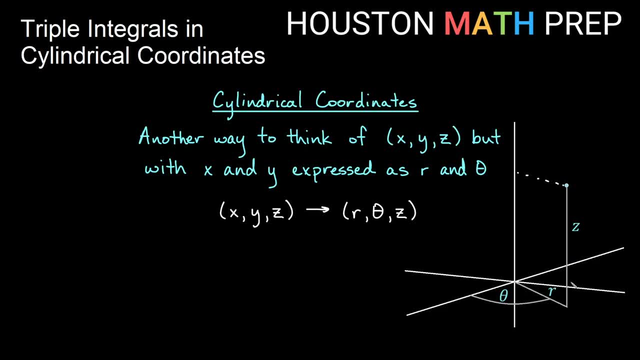 the positive x direction And, of course, z is going to be our height. If it's positive, it's above the xy plane, If it's negative it will be below. Remember from our video involving triple integrals in rectangular coordinates: our unit of volume for triple integrals is dv And we can write that as dxdydz or dzdydx. 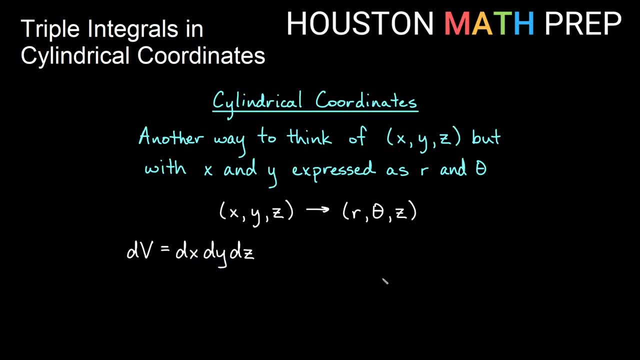 many different orders of this, But that's our unit of volume And if you think about replacing our x and y, we're not going to be able to use that unit of volume in cylindrical coordinates. We'll need to replace dxdy with rdrd theta. Remember that rdrd theta is your unit of area. 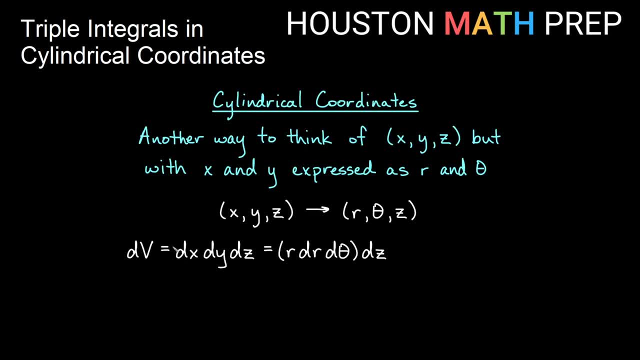 or a double integral in polar coordinates, And so we'll replace dxdy or dydx with rdrd theta, And so we end up with rdrd theta, dz. Or if we prefer to do our z component of our triple integral first, then we may write this as dzrdrd theta. So it really just depends. 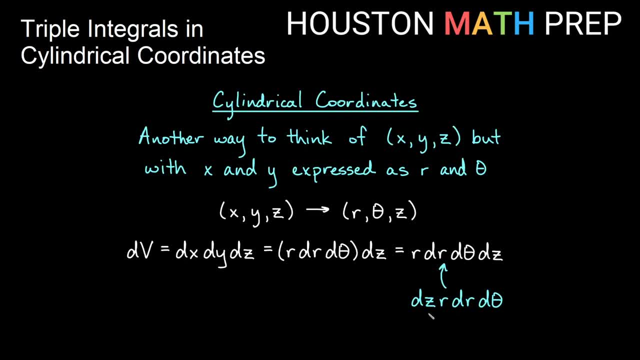 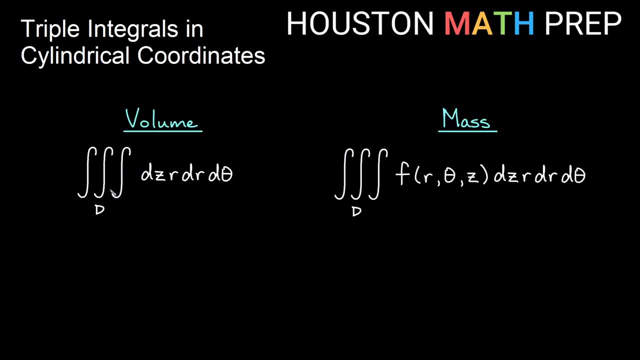 on the order of integration that you want to do In our video. here we're actually going to do this order: dzrdrd, theta. Remember that we can calculate volume with just simply a triple integral and our unit of volume. If we add some sort of function, that is not one. 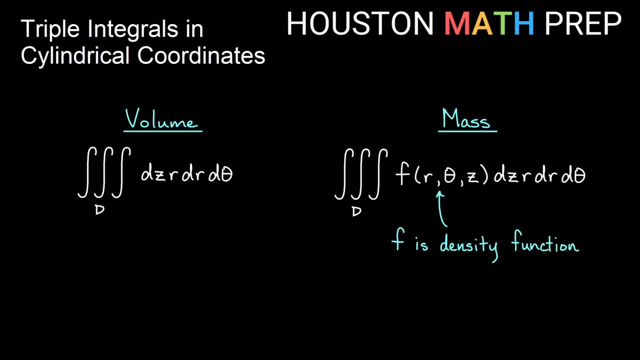 then we consider that to be a density function, And so we can calculate something like mass over a volume d. And remember that of course volume and mass are going to be the same when your function in here is one. So this is not strictly a volume triple integral It could be. 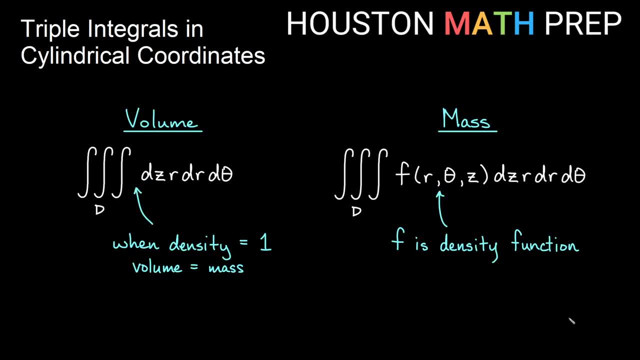 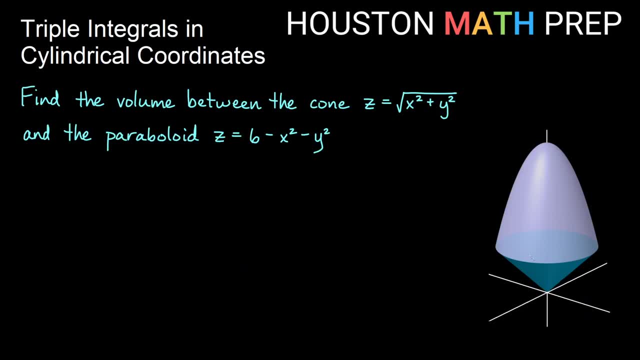 considered a mass integral if the density is one for your entire object there, Let's look at using a triple integral in cylindrical coordinates. Let's look at using a triple integral in cylindrical coordinates. We're going to find the volume between the cone z equals square root x squared. 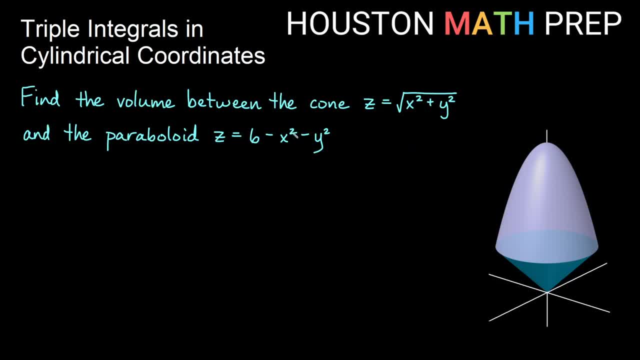 plus y squared, and the paraboloid z equals 6 minus x squared minus y squared. So if you think about the shadow that this is going to cast, the region in the xy plane that we used to think of in terms of double integrals, it's going to cast a circular region, And so a circular region, tells us, polar is. 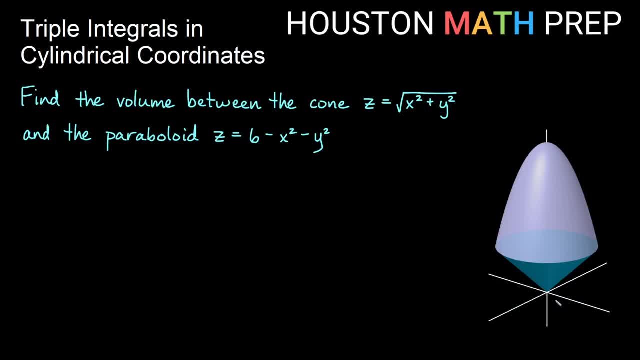 probably better suited for a multiple integral here than doing something in rectangular coordinates. So converting our x's and y's to polar and then setting up our triple integral for cylindrical coordinates is going to be the best thing to do here. So let's go ahead and set up our volume. Volume is going to equal triple integral. 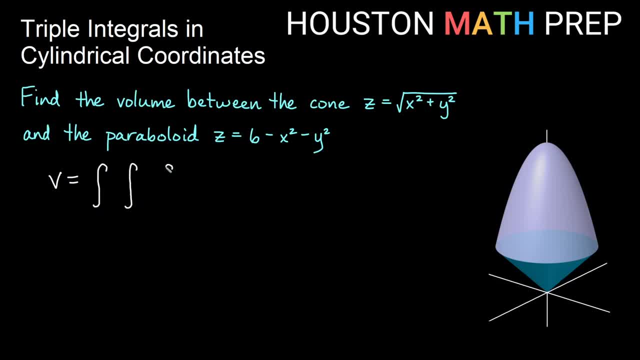 And I said I was going to go ahead and do this in terms of dz first. So we will have dz and then we will have r dr d theta, remember, is the unit for polar. Okay, so we'll need to first figure out our z bounds And remember the way that we'll do that is to just choose. 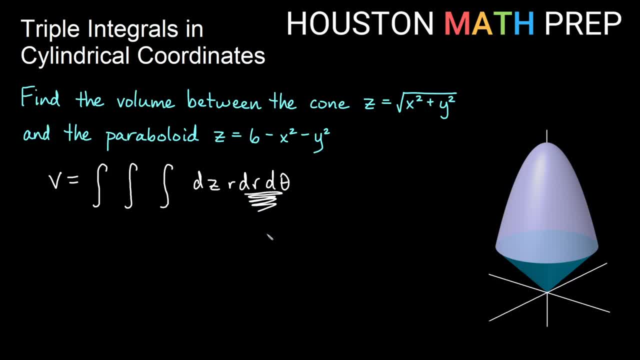 some r and theta. So we'll choose some point in the plane and draw through in the z direction. We'll have to multiply in our r later on, but we won't worry about that just yet until we're integrating. So I pick some point below my solid object here. Think about the shadow that this 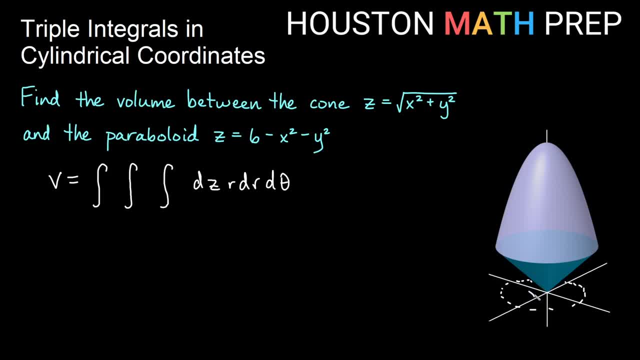 region casts in the plane, That's our region And I just pick some point in that region and I fix that and I draw through in the z direction. So if I draw through this point in the increasing z direction, think about what happens. I go into the region, I enter the region through the cone. 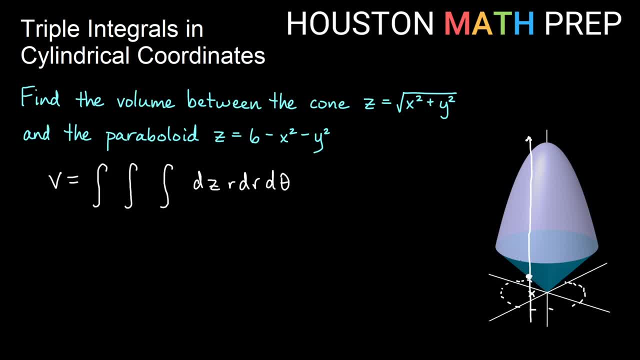 So that tells me that the cone is going to be my lower bound. So this is my lower bound for z And I come out of the paraboloid on the top. So this is going to be my upper bound for z. But now I don't just want to write it in terms of x and y in the formulas that I have here, because 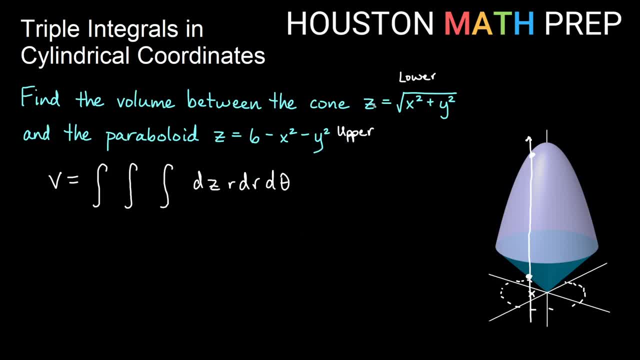 I need z's, r's and the thetas. So what we'll need to do is convert our equations for the cone and the paraboloid to a polar equation. So here, if you remember that x squared plus y squared equals r squared. So this is really the square root of r squared. 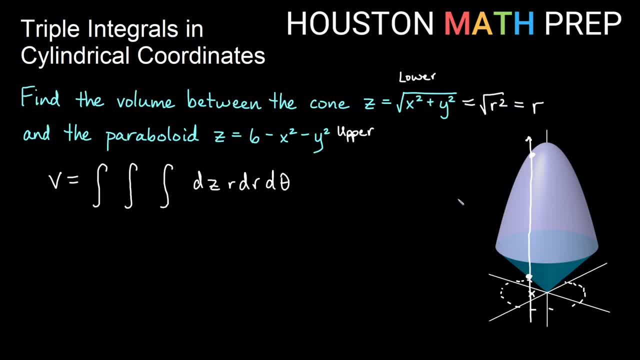 In other words, we're going to have just z equals r for our cone And our paraboloid. if you think of 6 minus x squared minus y squared, as 6 minus the quantity x squared plus y squared, then that's really going to be the same as 6 minus r squared. 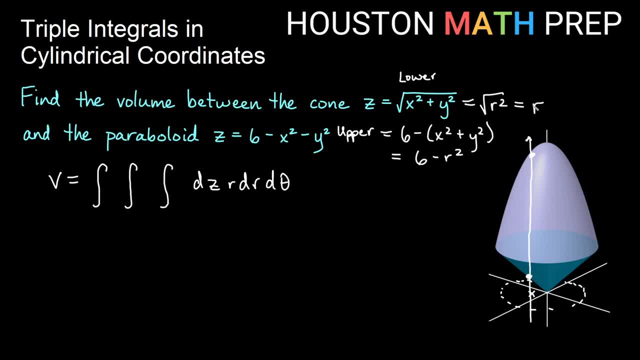 So my lower bound here is just going to be r. I go through the cone and its equation for z is r, And my paraboloid is my upper bound and its equation is 6 minus r squared. So those are our z bounds. We're integrating from r to 6 minus r squared. Now I have my r bounds next. 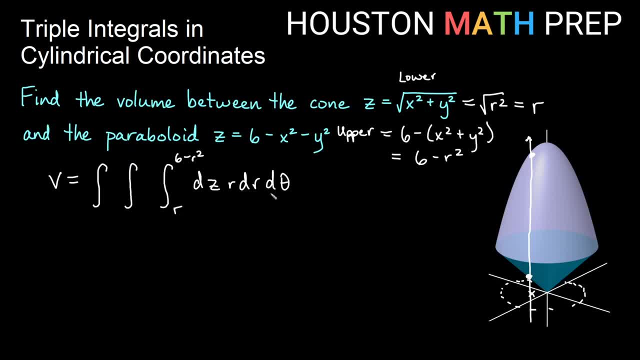 that I need to do here with this integral. So what I'll do? the only thing left outside of r is theta, So I'll fix some direction and I'll just draw through in the r direction in my region. So I want to go ahead and draw my region. Well, that's a circle, right? So if I draw my circular, 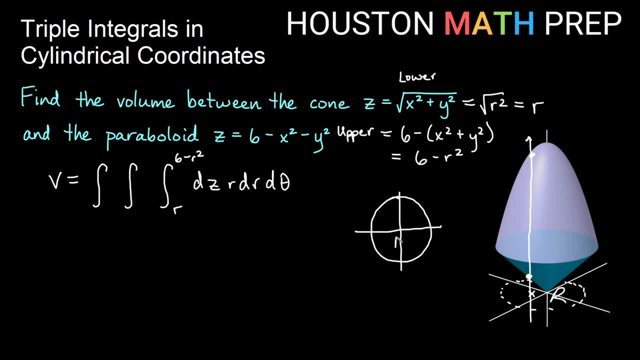 region that I have. so this region here is this picture. So if I just pick some theta and draw through in the r direction, So I will start at the pole, and if I just go out some direction, then that will look like that I will come out of the region here. 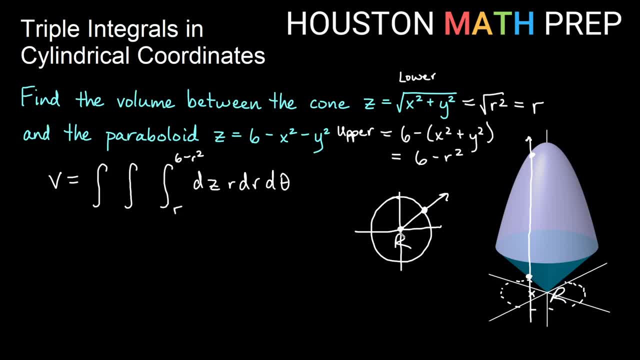 on the circle. So the question is: how big is this circle? right, I know the pole starting would be at r, equal to zero, but how far out is this, And the way we could figure this out, the size of this circle, the shadow that's cast from this would be: 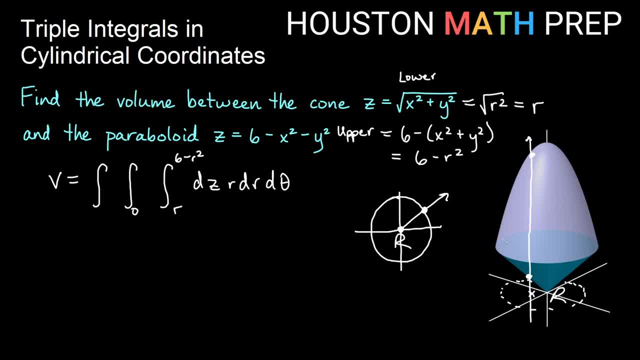 it's being cast from the intersection ring right, So that's where these things are equal to each other. So I could figure out the size of my circle, my r, whenever my cone r is equal to my paraboloid 6 minus r. squared, That would be my intersection value for r right. 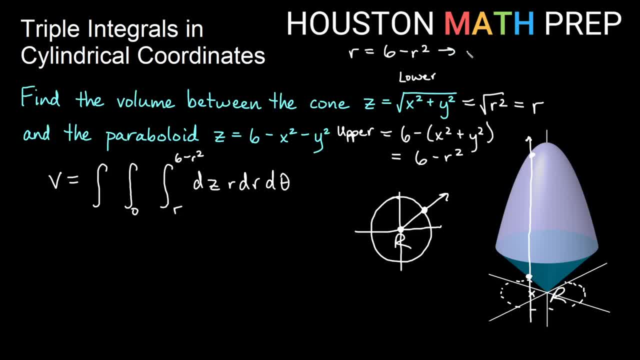 I get everything on one side, move everything to the left. maybe that would be r squared plus r minus 6, equal to zero. And if we do some factoring here we'll get r plus 3 and r minus 2 as the factors, equal to zero. And if I set both of these equal to zero, 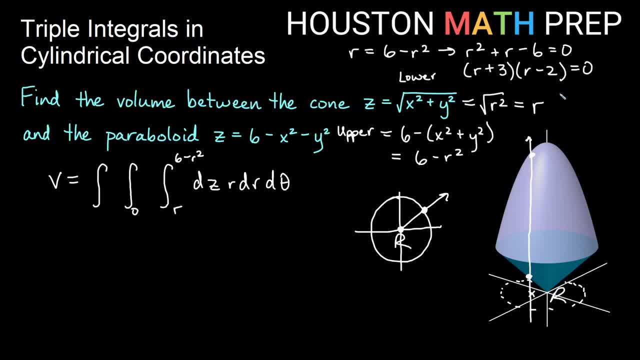 I think we'll look at the positive one and not the negative one. So this will tell me that r is 2. And so I know that my region that I'm trying to use to decide my dr d theta bound, has a radius of 2.. So, in terms of going out from the pole, how far do we go? We go out to a radius. 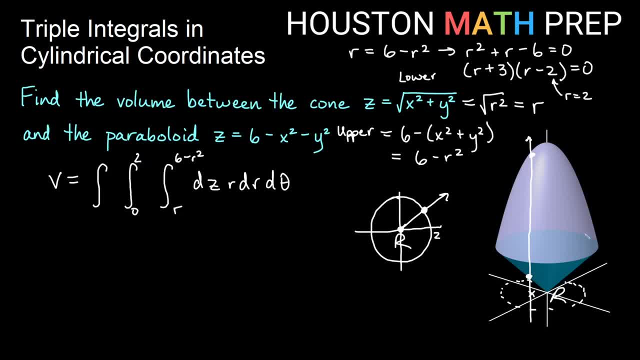 of 2 is our upper bound for r, And since we want the entire volume of between the cone and the paraboloid, not just say you know one side of it, then we're going to go all the way from zero to 2 pi, all the way around that object. So this is our triple integral in cylindrical coordinates. 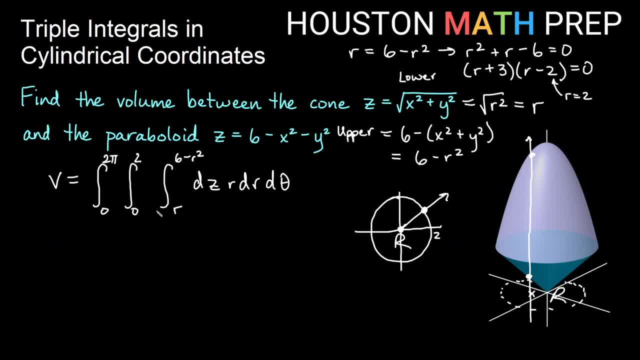 that represents the volume of this. Let's go ahead and start to work on this. Remember first that we will do our integral. So we'll go ahead and say that this is equal to the integral from zero to 2, pi integral from zero to 2.. And if I integrate dz, then I just get like I do in rectangular. 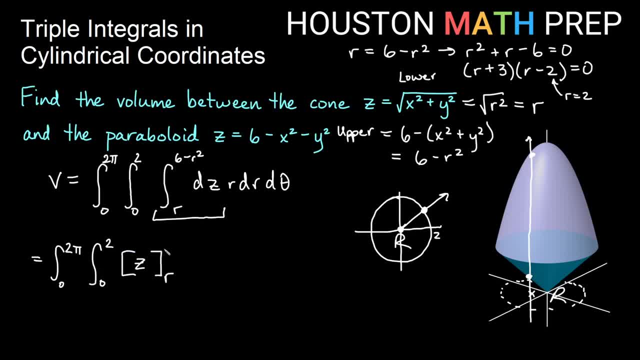 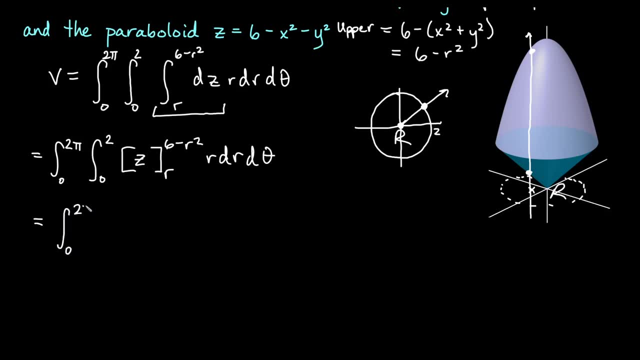 coordinates, triple integrals. I just get z. We'll integrate from r to 6 minus r squared, And we'll still have r dr d theta out here. Okay, now, if we plug in our bounds, what will happen here is we'll do the top minus the bottom, and then we're going to point something out here. 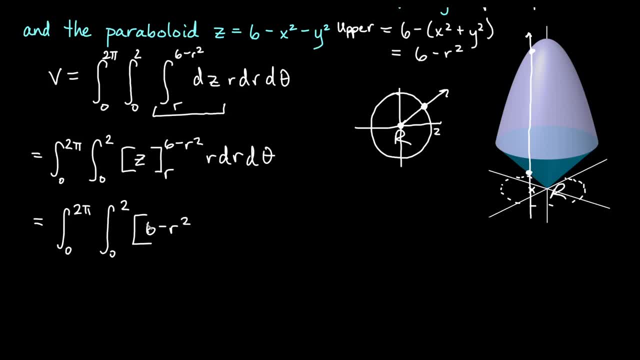 So we would get 6 minus r, squared minus r, and that would be what we would have, and we'd integrate that r dr d theta. Now this is the same integral that we would get if we set this volume up as a double integral. 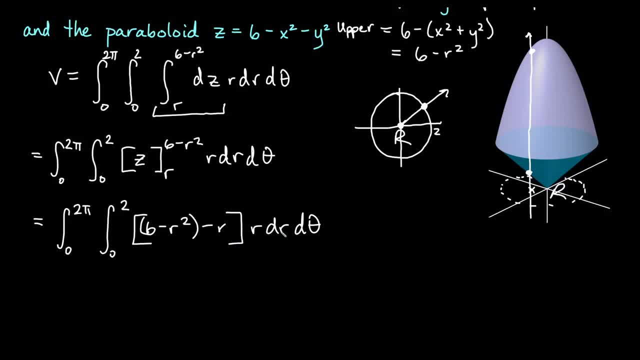 with our top function minus our bottom function, We would get this exact same setup, doing a double integral in just polar coordinates instead of a triple integral in cylindrical coordinates. We do need to learn to do these triple integrals, though, because we can't do something like a mass. 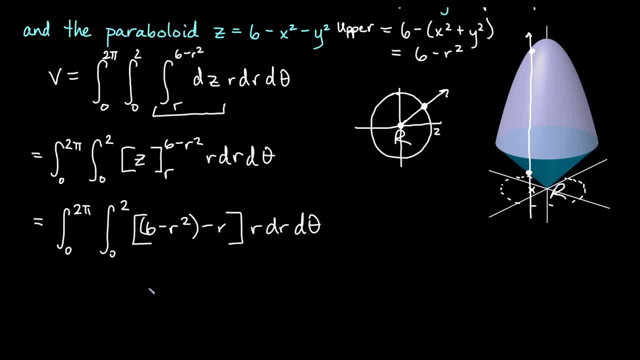 of a three-dimensional object very easily with a double integral and putting functions inside of it. So these triple integrals are going to be key for us to do things beyond just volume. Okay, let's go ahead and distribute our r and then we can move on from here with our 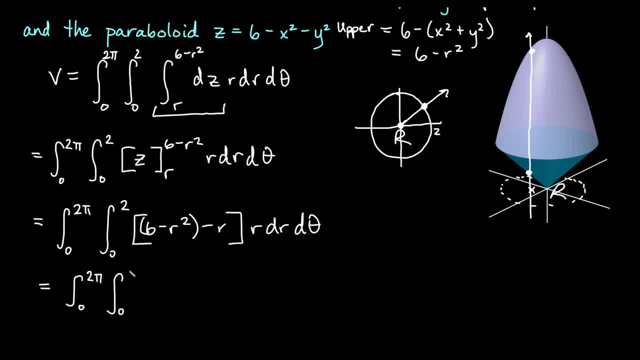 dr step. So we'll have from 0 to 2 pi and 0 to 2 and then distributing r, I will get 6r minus r cubed minus r squared and we'll integrate that dr and save our d theta for last. 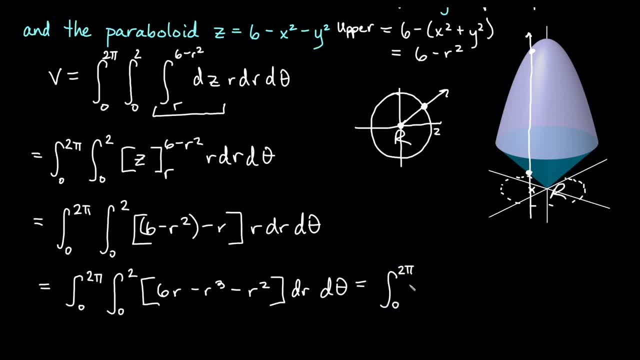 So we'll keep our 0 to 2 pi and integrating this dr we will get 3r squared minus one-fourth r squared minus one-fourth r squared to the four minus one-third r cubed. We'll evaluate that from 0 to 2. 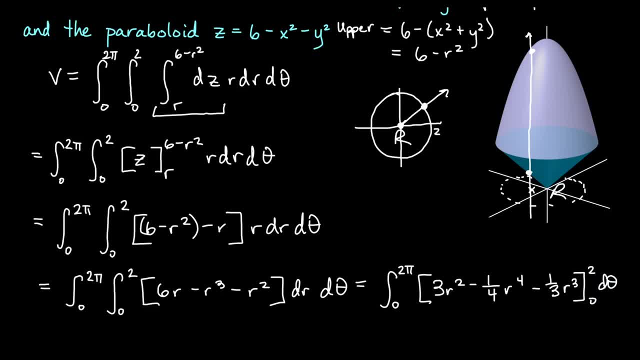 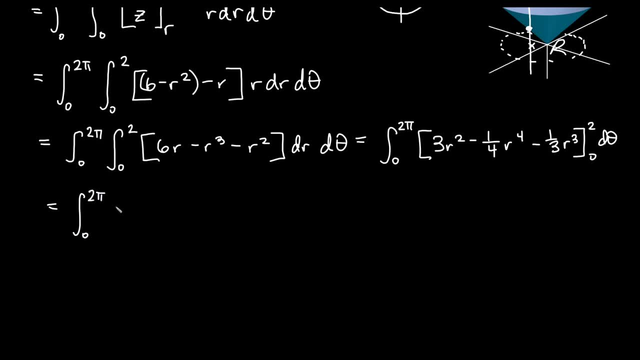 and then we'll integrate at the end d theta. Okay, let's go ahead and plug in our bounds, so we will get the integral from 0 to 2. pi of plugging in 2 everywhere I would get 3 times 2. squared would be 4 minus one-fourth times 2 to the 4 would. 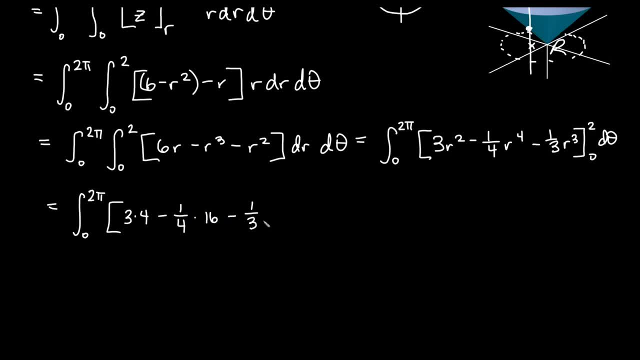 be 16 minus one-third 2 cubed would be 8, so get 8 times a third there. if I plug in 0 everywhere, I'll get 0 and 0 and 0, so minus 0 there, and then we'll have d theta. so this will then give us. 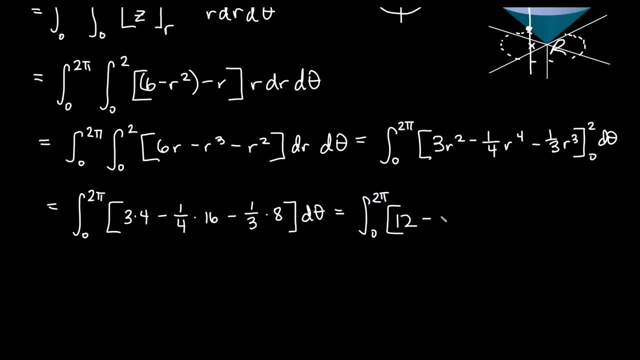 if I simplify this stuff, we'll have 12 minus 4 minus 8 thirds, so this will be then integral of 0 to 2 pi. so we have 8 minus 8 thirds. think of this: 24 over 3 minus 8 over 3, we have 16. 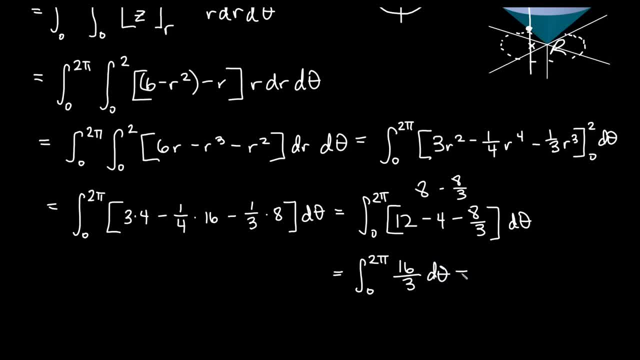 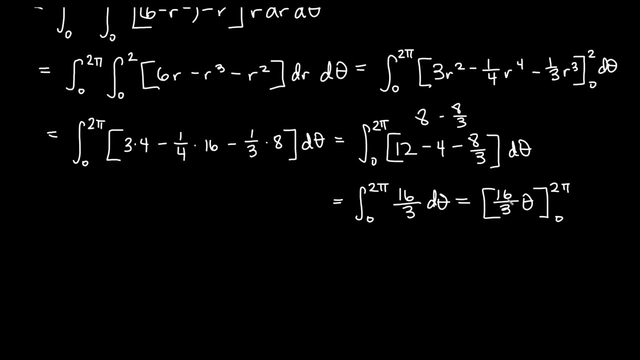 over 3 in here, integrating that d theta. and then if we integrate d theta we will just get 16 over 3 times theta, evaluated from 0 to 2 pi, and if I plug in 2 pi, 16 over 3 times 2 pi. 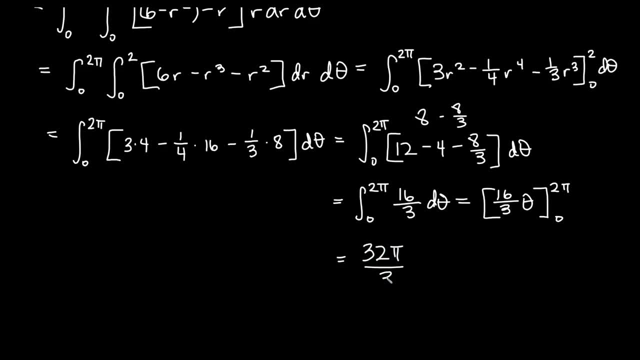 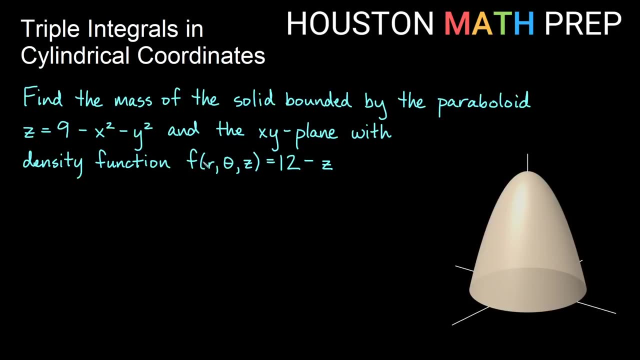 is going to give me 32 pi over 3, and if I plug in zero then I'll get minus zero. so we just end up with 32 pi over three for our volume here. All right, let's do another example with mass that we couldn't do with a double integral. so find the mass of the solid bounded by the paraboloid z. 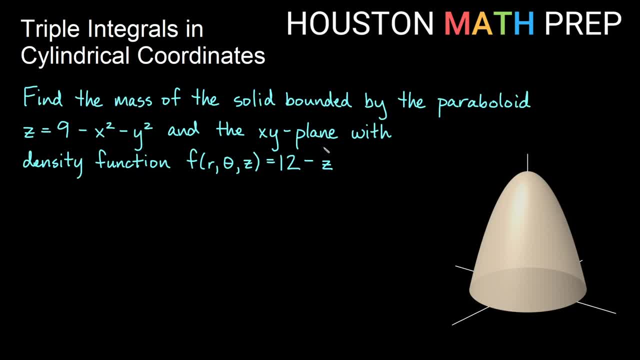 equals nine minus x squared minus y squared and the xy plane. so the bottom is the xy plane. we have a density function here. in terms of cylindrical coordinates it's 12 minus z. so think about what's happening. as z is big, then we get less density, right with a big number. think about like: 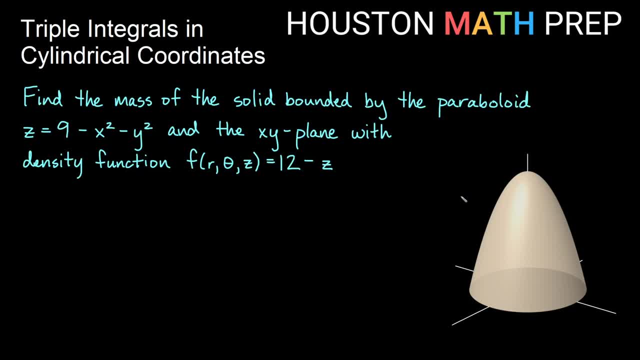 12 minus 9. here the density would be 3 at the very top. but as we get further and further down the object, this z, is going to get smaller. so we'd get 12 minus something smaller. we'd get a larger value for the density at the bottom than at the top. so this thing is heavier right at the bottom. 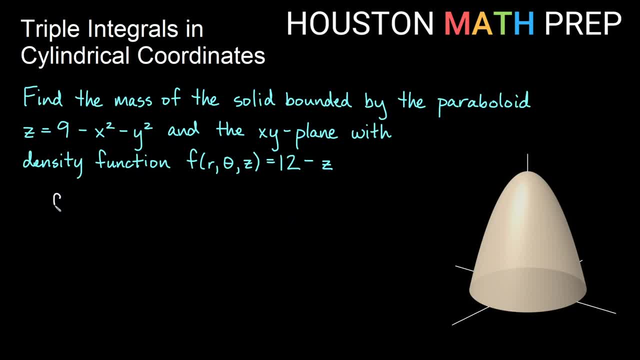 than it is at the top of the object. okay, let's go ahead and set up our triple integral. we'll need our density function inside of the triple integral to give us the mass. so i will have a function of 12 minus z in there, and i'm going to go ahead and set this up in the same order just to get. 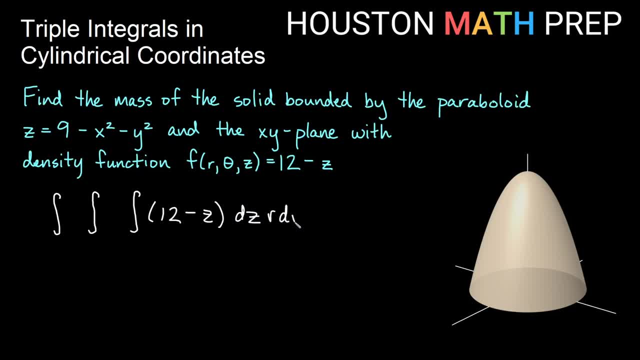 good practice, like we had on the last one- dz, r, dr, e, theta- and i'll need to choose my z bounds first. so remember first i'm going to just fix some point in the polar plane and draw through in the increasing z direction. so if i think about picking some point in the base and i draw through in the z direction, 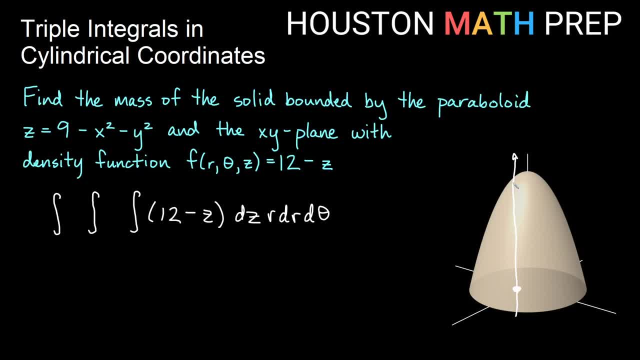 increasing. i enter at the plane and i come out the top surface of the paraboloid. the plane is going to be z equals zero. the paraboloid is going to be z equals this equation: nine minus x squared minus y squared, except in terms of cylindrical or 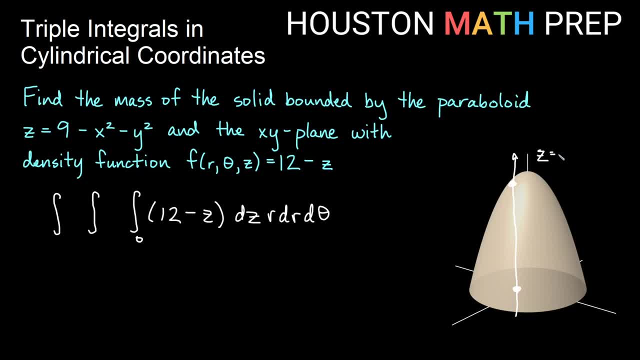 in polar right, we would think of this as z equals 9 minus r squared, so we'll actually have an upper bound of 9 minus r squared for our paraboloid. okay, now i need r bounds. so if i think about my region here, i have a circle again and my circle. i just need to know how big it is, and that's going to. 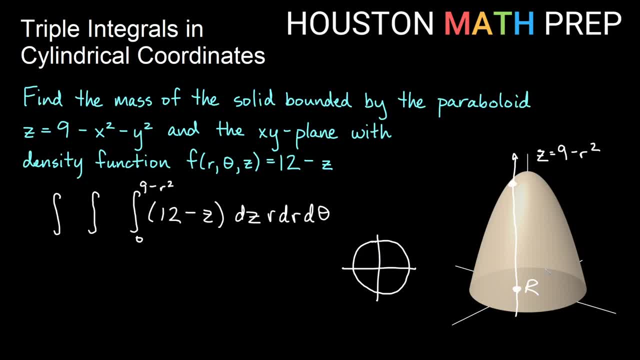 tell me, my r bounds right. so how big is this? well, this circle is where the paraboloid meets the, the axis right, in other words, when the z value is zero. so if this circle is zero equals nine minus r squared. then r squared is equal to nine and i think our radius is three, right. so our 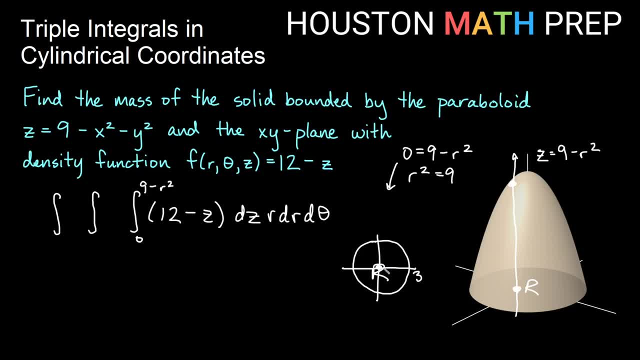 region that we have. if we're going out from the pole to find our r bounds from here out to the circle, then that would be from an r value of zero out to an r value of three. so our r bounds are going to be from zero to three, and then we want the entire paraboloid, so we'll go all the way. 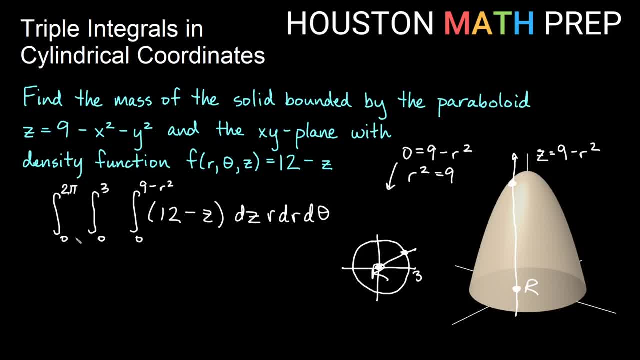 around from zero to two pi. so just our triple integral, dz, r, dr, d, theta would be the volume. but now we're including the density function to calculate the mass of this object here. so we will have zero to two pi, zero to three. and now we don't just get z whenever we integrate dz here, because 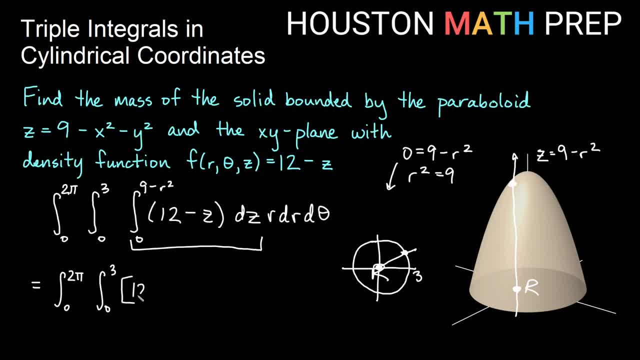 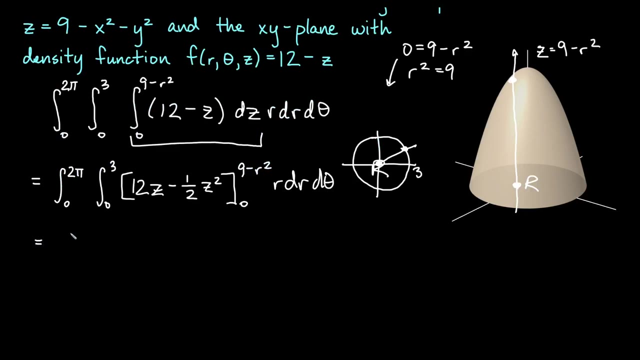 we have function twelve minus z, so in here we will get twelve z minus one half z squared. we will have to plug in our bounds zero to nine minus r squared, and then we'll have r dr d theta in the steps that follow after this. all right, let's plug in our bounds, so we will get from zero to two pi and zero to three. 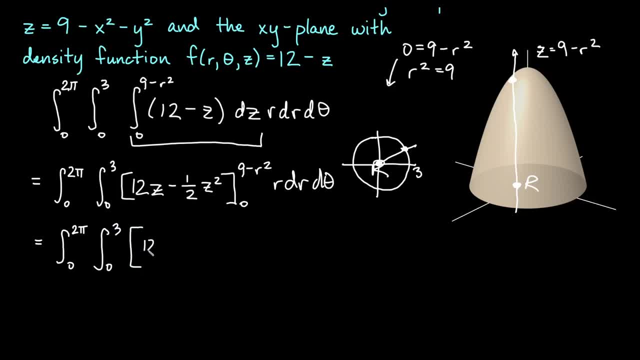 and plugging in, we will get twelve times nine minus r squared, minus one half times now z squared. so we'll get nine minus r squared, all squared minus. when we plug in zero, that will just give us zero for everything, and then we'll worry about r dr d theta after all that okay. so we need to do some. 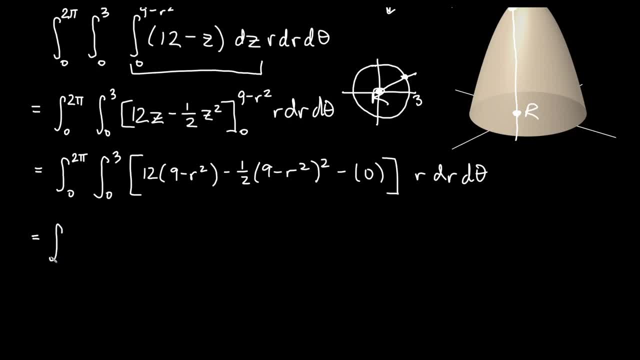 distributing. so we'll have from zero to two pi, we'll have from zero to three, and then we need to distribute in here. so 12 times 9, that'll be 108 minus 12, r, squared minus. i'm going to keep the one half. let's distribute this perfect square first. 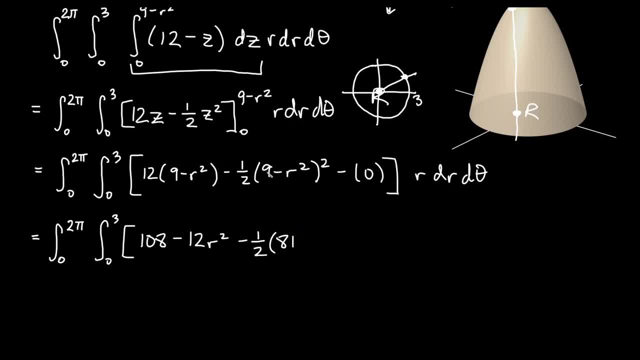 so 9 times 9 would be 81.. i'd get minus 9 r, squared minus another 9 r, squared minus 18 r, squared plus 8 r squared minus 9 r squared minus 18 r squared plus r-squared times, r-squared r to the 4.. 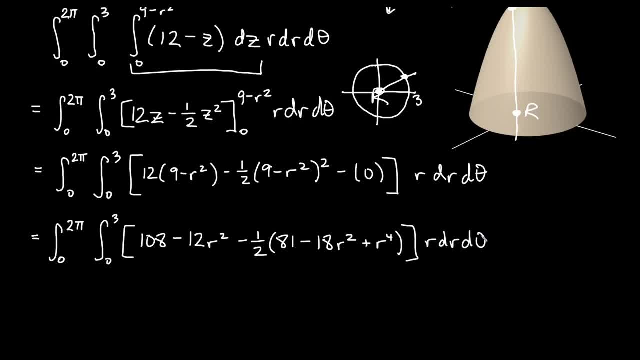 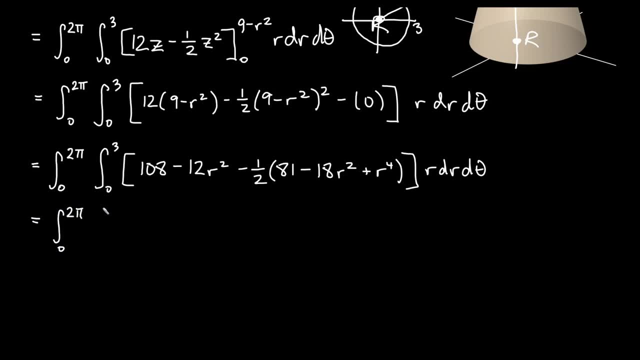 We have r dr d theta on the outside. We'll go ahead and distribute our half and I think you can see life is not happening in whole numbers here and that's certainly okay. So we will get 108 minus 12r-squared minus 81 over 2. 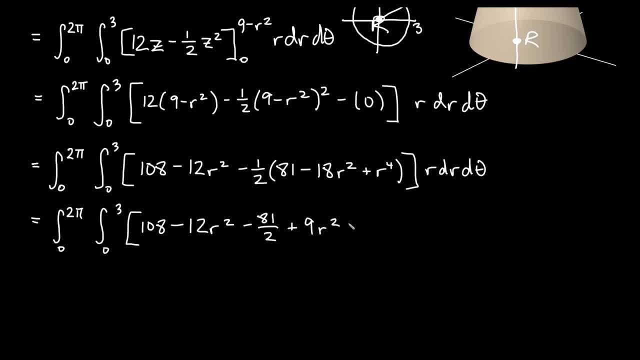 plus 9r-squared, minus 1 half r to the 4. r, dr d theta. Okay, so I'm going to go ahead and think of this. so I get a common denominator: This is 216 over 2.. So when I write this down and combine my like terms: 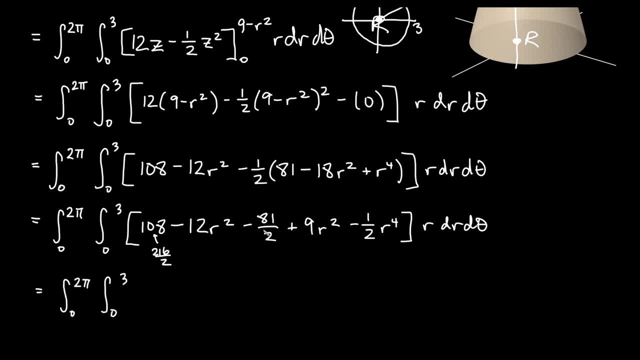 I'll just have one thing here. So 216 over 2 minus 81 over 2, that will give us 1. 35 over 2.. I'll have negative 12r-squared and plus 9r-squared. 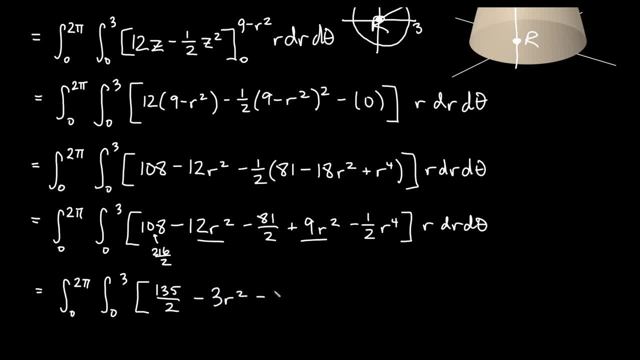 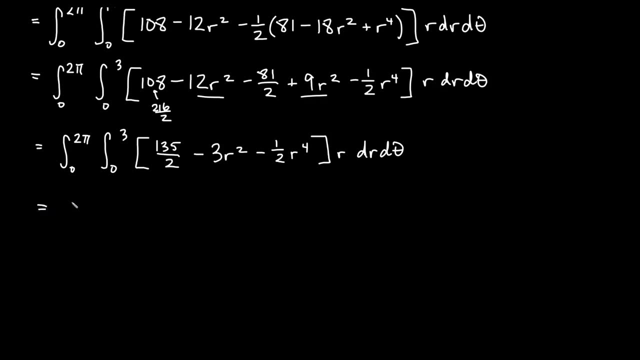 That would be minus 3r-squared, minus 1 half r to the 4.. Still And now, still to go, I need to distribute my r. I have an r out here. We don't want to forget that. It's definitely needed. 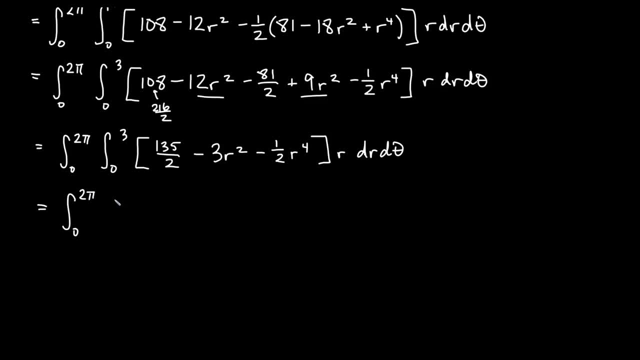 So integral from 0 to 2 pi, we're getting there Integral from 0. To 3, that will be 1, 35 over 2 times r minus 3r-cubed, minus 1 half r to the 5.. 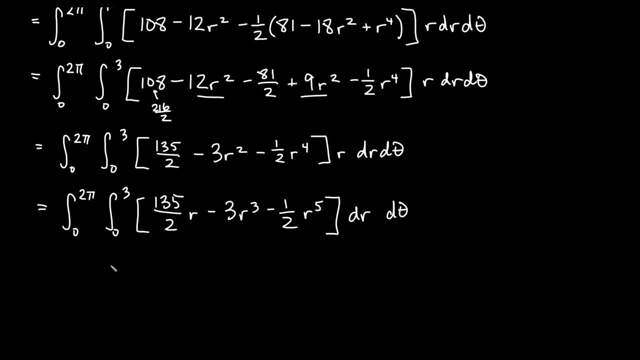 We'll integrate dr next and then d theta will be last. Okay, so I have to integrate. Just be careful with our numbers here. So if we integrate this power rule, we divide by 2 and the power goes up by 1.. 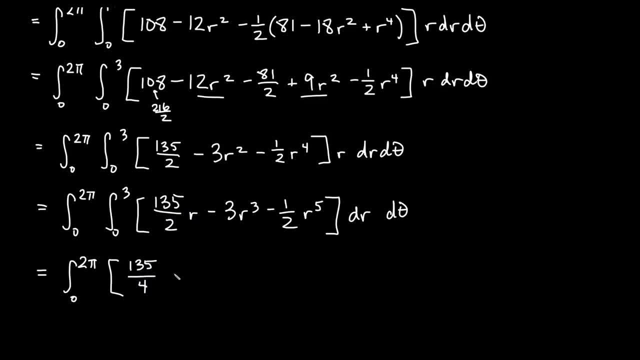 So we'll get 1.. 35 divided by 2 gives us over 4r-squared, minus r to the 4.. We get an over 4 here, So 3 over 4, r to the 4. This one here minus I would get r to the 6 over 6.. 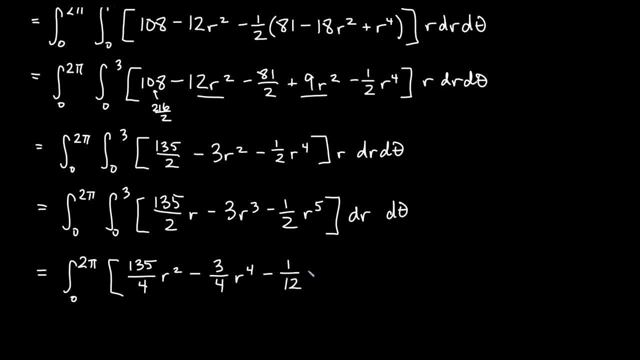 I already have a 2 there, So that will make 1 over 12r to the 6. We'll evaluate from 0 to 3. And then we'll have to do d theta at the end. Okay, now our 0s will give us: 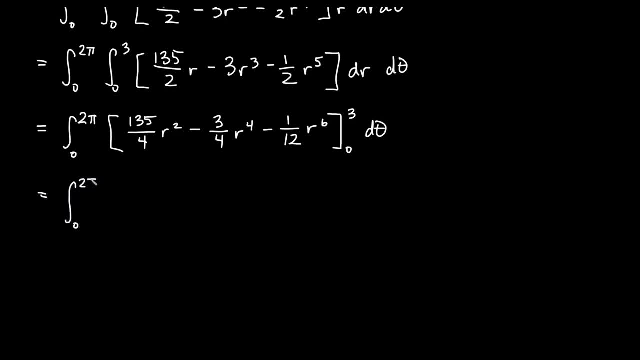 0 for each term, So it's just the 3 that we really need to do here. Let's go ahead and plug in our 3s, So we'll get 1, 35 over 4 times 9,, 3 squared. 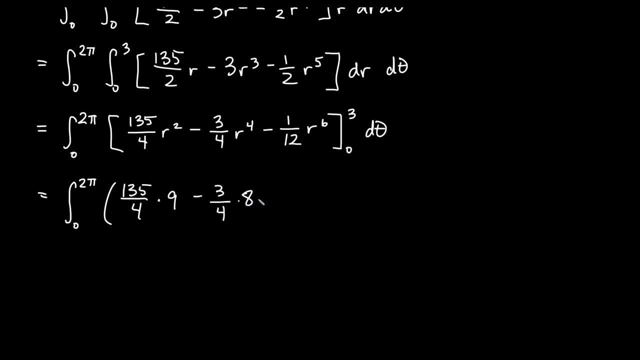 minus 3 over 4 times 3 to the 4 is 81, minus 1 over 12, 3 to the 6 is actually 729.. Okay, now I'm going to go ahead and multiply and then do some things here. 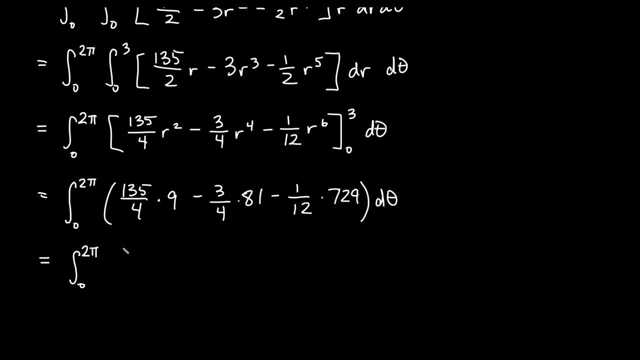 That will make this maybe just a little bit easier to do by hand. So 9 times 1, 35, that's going to be 1215 over 4, minus 3 times 81 on the top will be 243 over 4.. 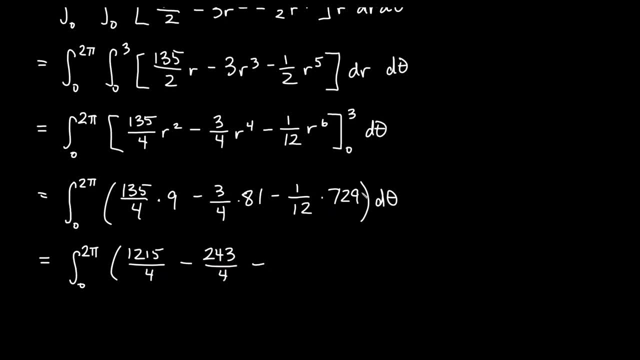 You can see we have nice over 4s here. I have an over 12, but if I reduce this top and bottom by 3, and that becomes 243 on top and a 4. So I get another minus 243 over 4 d theta. 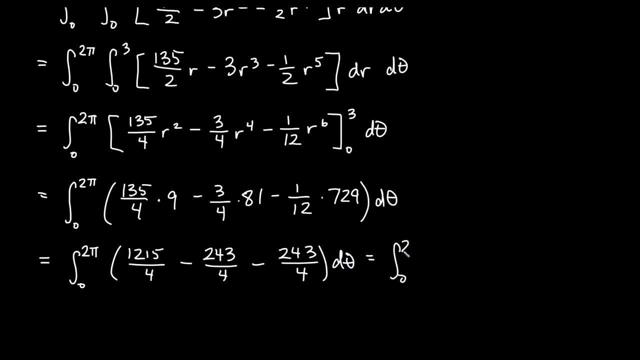 And now let's just combine So we'll have 0 to 2 pi and then this amount here: 1215 minus 243 minus 243.. That's going to give us 729 over 4.. And we'll integrate that d theta. 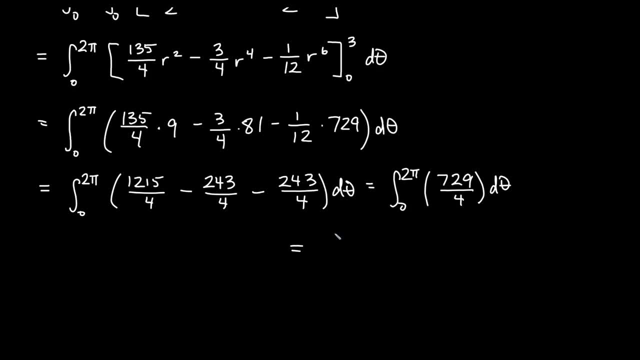 And let's go ahead and do that. We're almost there. So if I integrate that, of course I just get 729 over 4 theta. That's easy, at least right. And then plugging in from 0, to 2 pi, the 0 is not going to give me anything if I plug that in for theta. 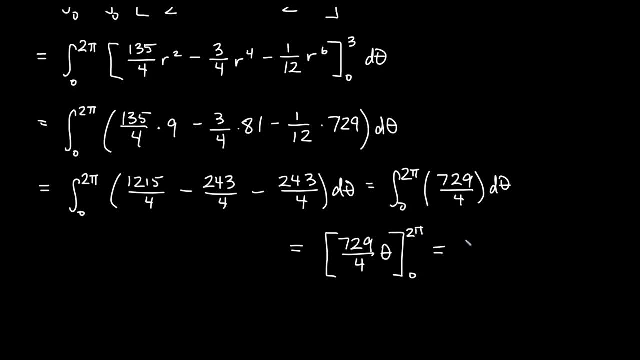 If I plug in 2 pi here, the 2 will reduce with the 4. So we'll get 729 pi over 2. as our remember this was mass, because we had a density function over our volume. Okay, hopefully this gives you a good idea of how cylindrical coordinates. 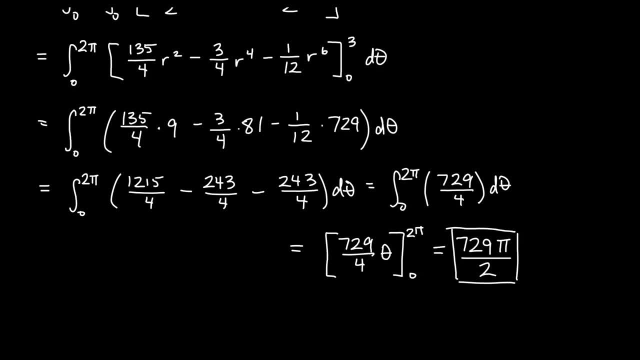 relate to polar coordinates, changing to r's and theta's, using r, dr, d, theta, But now with the dz component and a third integral. thanks for watching everybody. We'll see you in the next video.